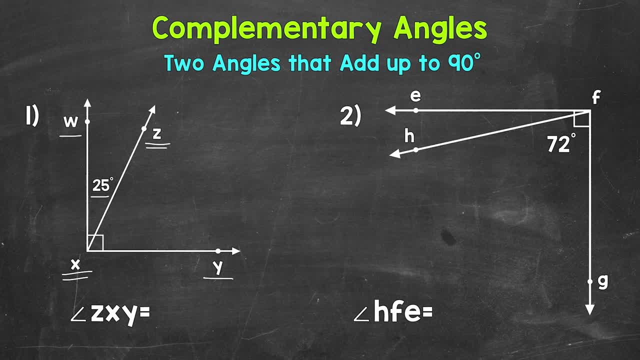 well, 25 degrees plus what equals 90 degrees. Well, 25 plus 65. So our missing angle measure is going to be 65 degrees. Angle Z, X, Y equals 65 degrees. If you can figure these out mentally, that works for sure. 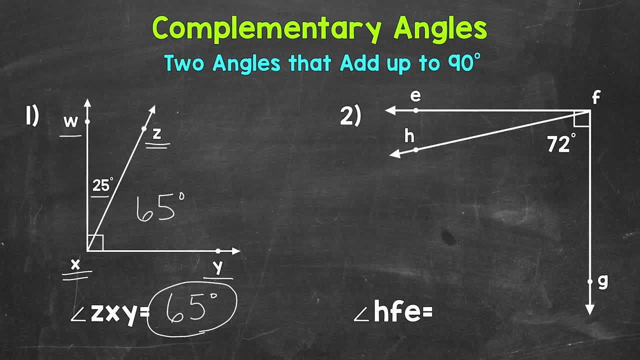 But if not, that's fine too, What we can do. we can take the 90 degrees that we know these two angles are going to add up to, So let's write 90 degrees and we can subtract the angle measure that we are given. 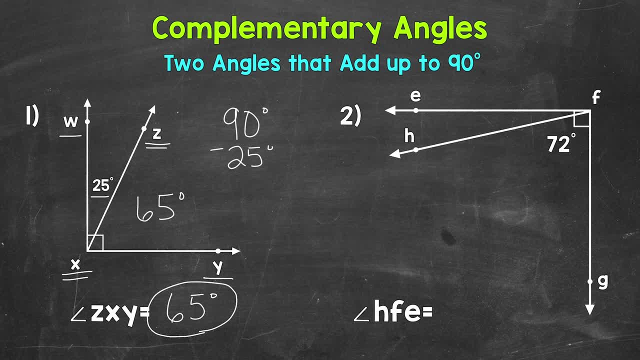 So 90 degrees, 90 degrees minus 25 degrees. Now we're ready to subtract, So we have 0 minus 5.. We need to borrow. Let's borrow from the 9 here, And we have 10 minus 5, which is 5.. 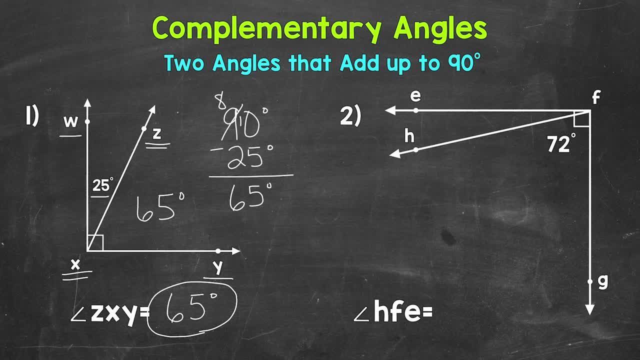 And then 8 minus 2 is 6.. So we get 65 degrees that way as well. Again 90 degrees, because we know the two angles are going to add up to 90 degrees And we can subtract. We can subtract the given angle measure in order to get that missing angle measure. 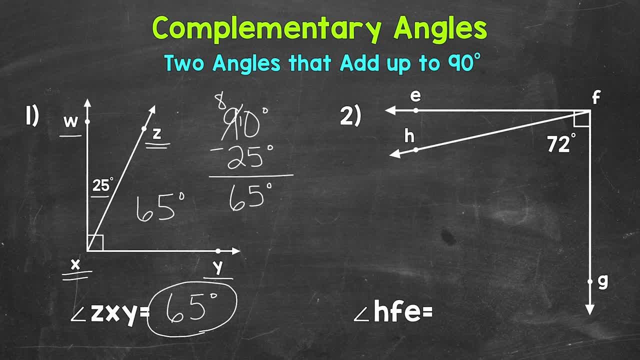 We can also check to see if our answer is correct by adding our two angles and then seeing if it equals 90 degrees. So let's double check here. We can do 65 degrees plus 25 degrees. If that equals 90, then we're good to go. 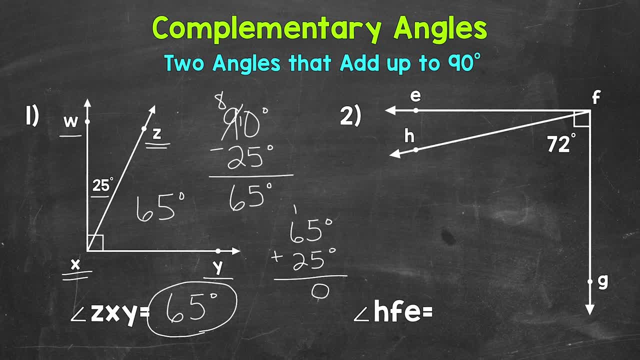 5 plus 5 is 10. So we have a 0 here. Vary the 1. 1 plus 6 is 7. Plus 2 is 9.. So those two angles equal 90. We have the correct answer there. 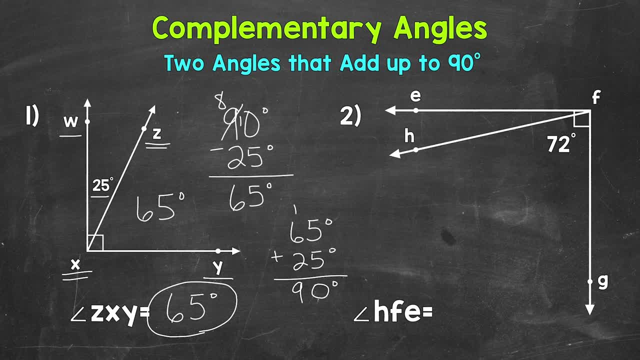 The missing angle. there is 65 degrees. Let's try another example here and move on to number 2, where we have a given angle measure of 72 degrees. So angle GFH equals 72 degrees. We need to figure out angle H. 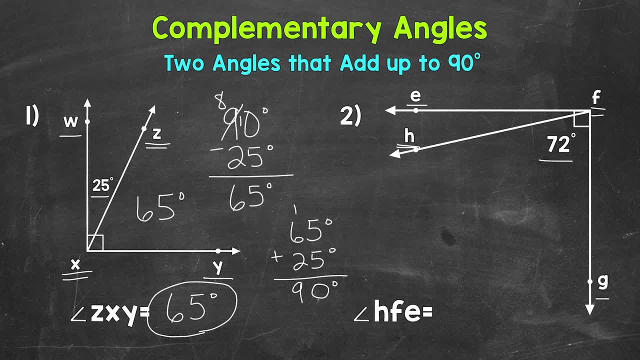 We need to figure out angle HFE. So let's do 90 degrees. We have complementary angles here, so we know they are going to equal 90. And we are going to subtract the given angle measure. Now again, if you can figure this out mentally, that's great. 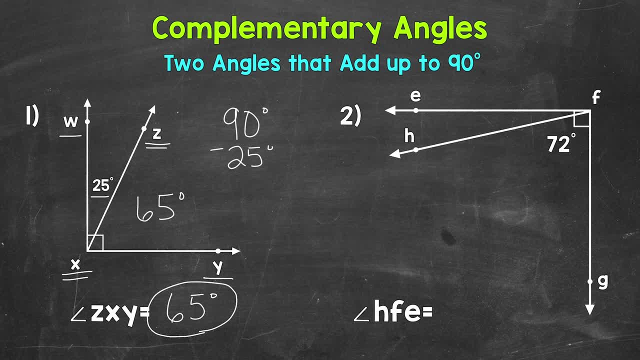 So 90 degrees, 90 degrees minus 25 degrees. Now we're ready to subtract, So we have 0 minus 5.. We need to borrow. Let's borrow from the 9 here, And we have 10 minus 5, which is 5.. 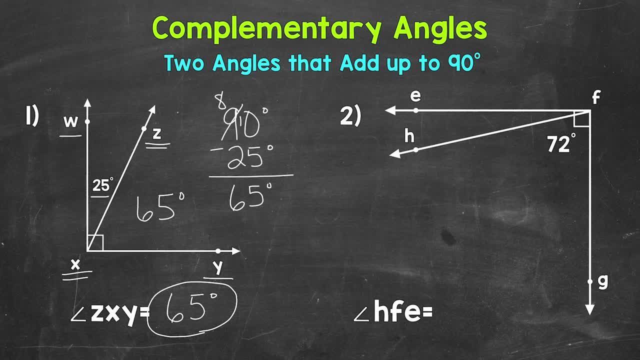 And then 8 minus 2 is 6.. So we get 65 degrees that way as well. Again 90 degrees, because we know the two angles are going to add up to 90 degrees And we can subtract. We can subtract the given angle measure in order to get that missing angle measure. 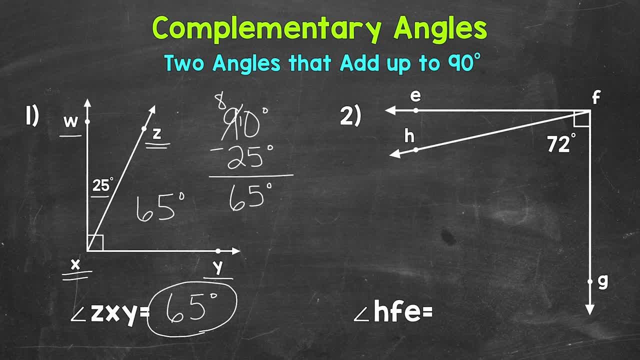 We can also check to see if our answer is correct by adding our two angles and then seeing if it equals 90 degrees. So let's double check here. We can do 65 degrees plus 25 degrees. If that equals 90, then we're good to go. 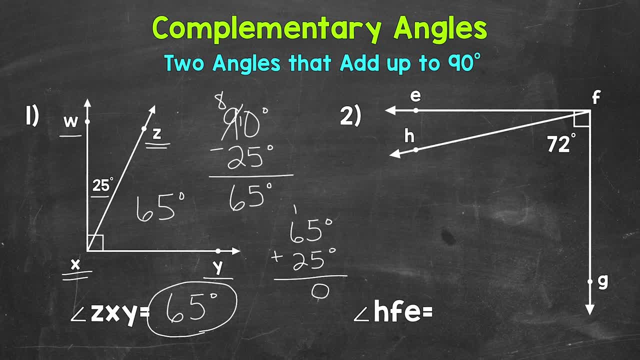 5 plus 5 is 10. So we have a 0 here. Vary the 1. 1 plus 6 is 7. Plus 2 is 9.. So those two angles equal 90. We have the correct answer there. 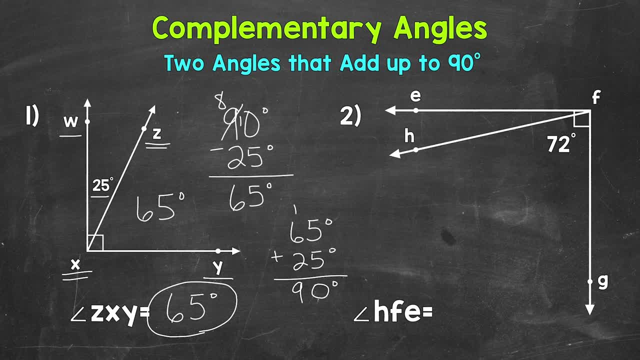 The missing angle. there is 65 degrees. Let's try another example here and move on to number 2, where we have a given angle measure of 72 degrees. So angle GFH equals 72 degrees. We need to figure out angle H. 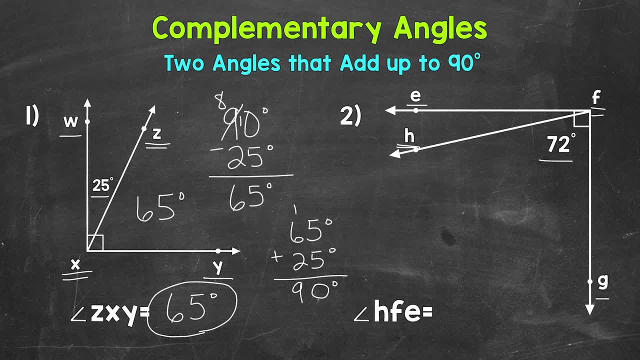 We need to figure out angle HFE. So let's do 90 degrees. We have complementary angles here, so we know they are going to equal 90. And we are going to subtract the given angle measure. Now again, if you can figure this out mentally, that's great. 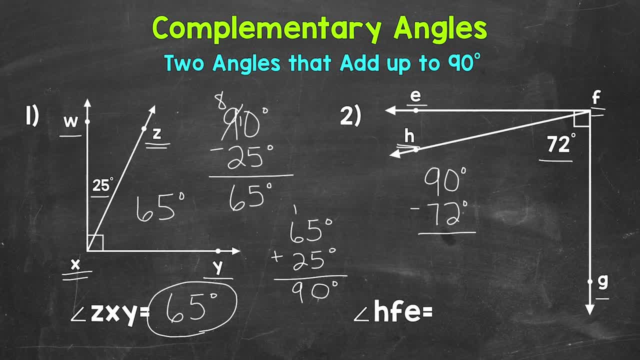 That works, But if not, that's fine too. We can always write out a subtraction problem to find that angle. So we have 0 minus 2.. Let's borrow: We have 10 minus 2, which is 8.. 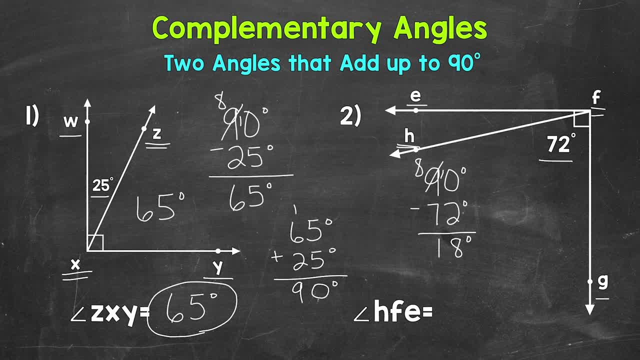 And then 8 minus 7 is 1.. So our missing angle angle HFE is going to be 18 degrees. Let's double check to make sure So we'll do 72 degrees plus 18 degrees. Make sure it equals 90.. 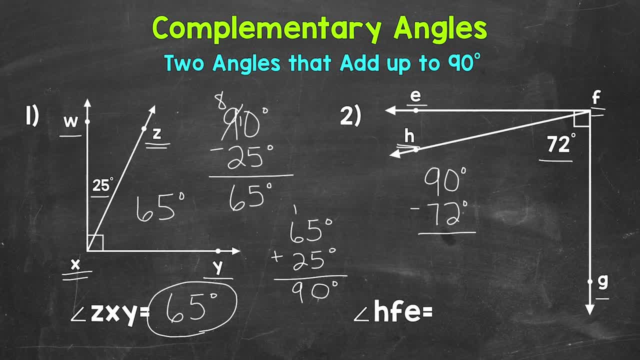 That works, But if not, that's fine too. We can always write out a subtraction problem to find that angle. So we have 0 minus 2.. Let's borrow: We have 10 minus 2, which is 8.. 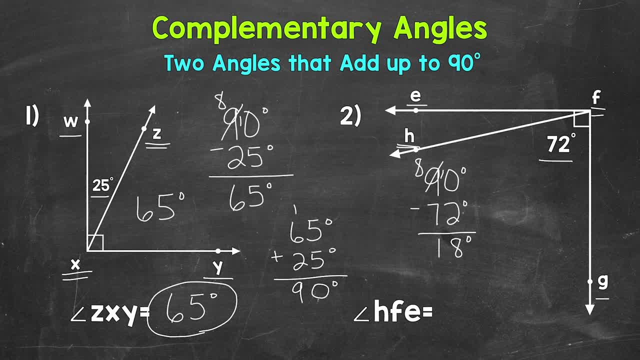 And then 8 minus 7 is 1.. So our missing angle angle HFE is going to be 18 degrees. Let's double check to make sure So we'll do 72 degrees plus 18 degrees. Make sure it equals 90.. 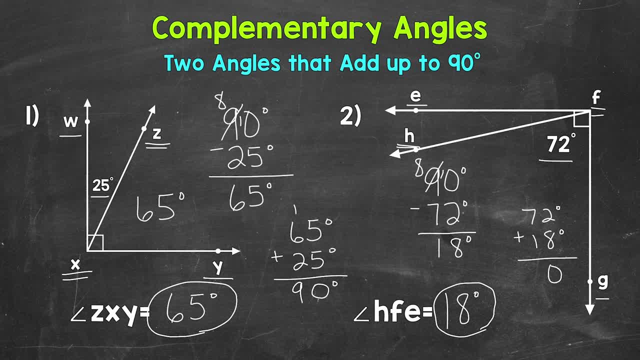 2 plus 8 is 10.. So let's put our 0.. Carry the 1. And then 1 plus 7 is 8.. Plus 1 is 9.. So those two angles do in fact equal 90.. 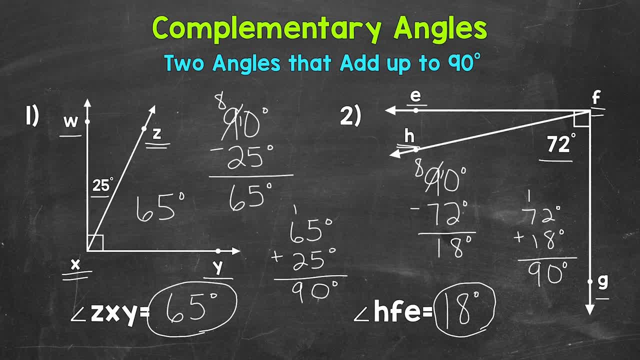 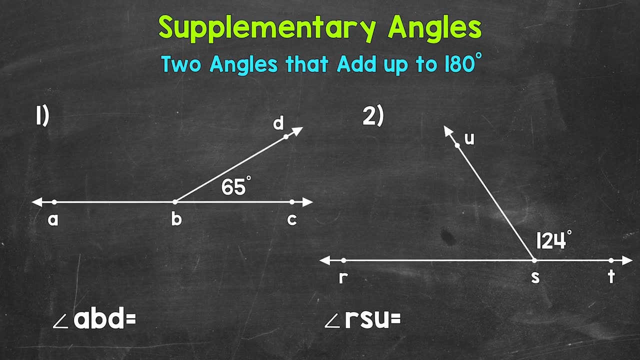 We have the correct angle measure for HFE 18 degrees. So there's an explanation of complementary angles. Let's move on to supplementary angles Now. supplementary angles are two angles that add up to 180 degrees, And a 180-degree angle is one angle. 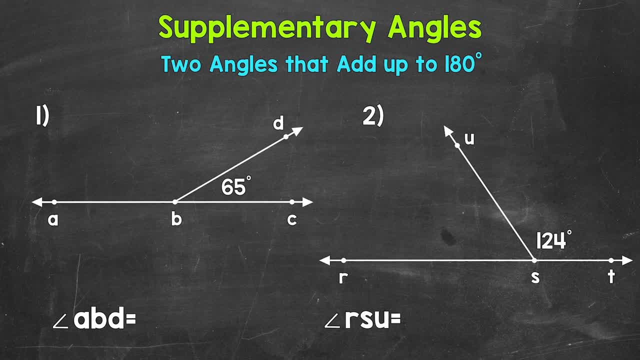 And a 180-degree angle is going to make a straight line. So if the sum of two angles is 180 degrees, they are supplementary. Let's jump into our examples where we have supplementary angles but one of the angles will be unknown or missing. 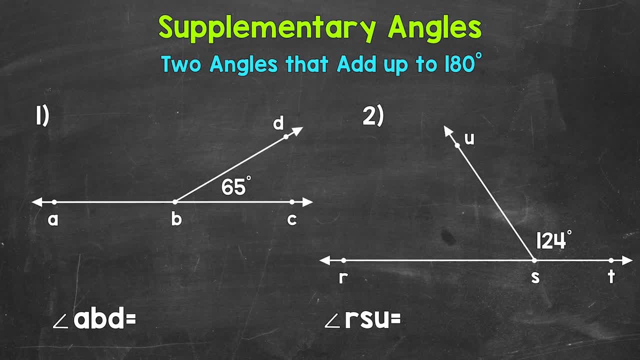 And we need to find that missing angle measure. For number 1, we have a given angle measure of 65 degrees, So angle DBC equals 65 degrees. So we need to find the missing or unknown angle. We are going to look for angle ABD. 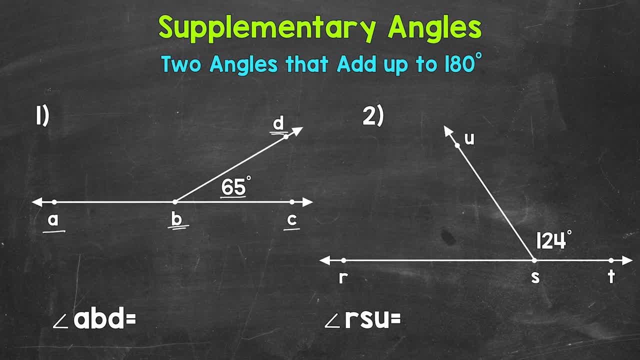 Now we know that the sum of these two angles is going to be 180 degrees. They are supplementary angles, So we need to think We have 65 degrees And then we need to add what to get to 180 degrees. 180 degrees: 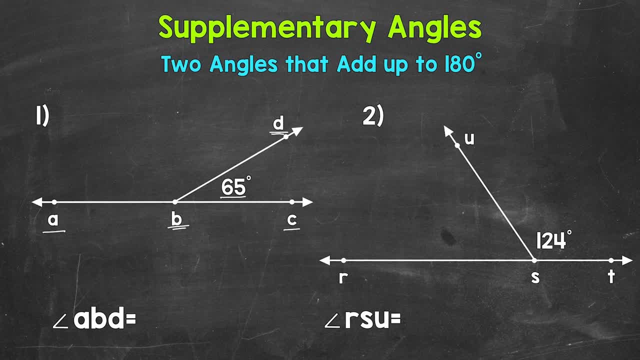 If you can figure these out mentally, that works for sure, But if not, that's fine too. So what we can do, we can take the sum of these two angles, which we know is going to be 180 degrees, So we will write 180 degrees. 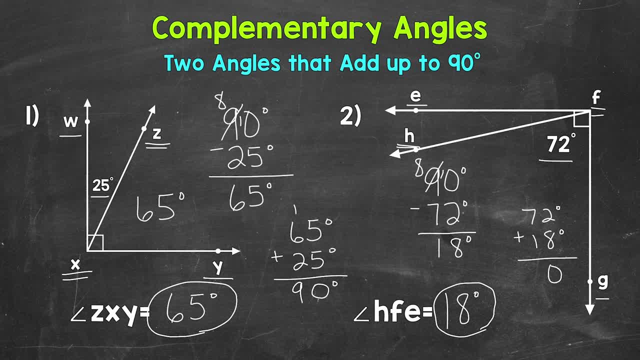 2 plus 8 is 10.. So let's put our 0.. Carry the 1. And then 1 plus 7 is 8.. Plus 1 is 9.. So those two angles do in fact equal 90.. 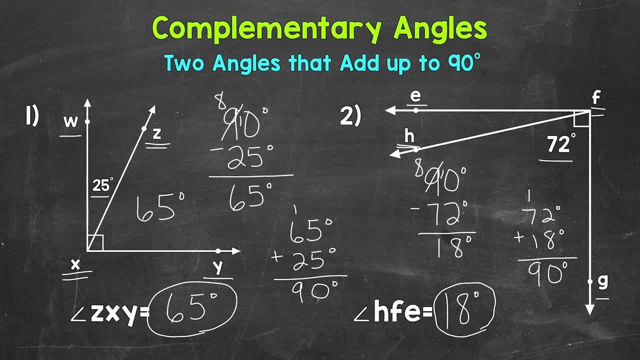 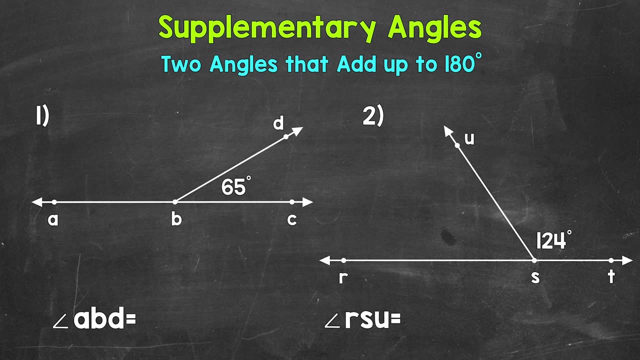 We have the correct angle measure for HFE 18 degrees. So there's an explanation of complementary angles. Let's move on to supplementary angles Now. supplementary angles are two angles that add up to 180 degrees, And a 180-degree angle is 1.. 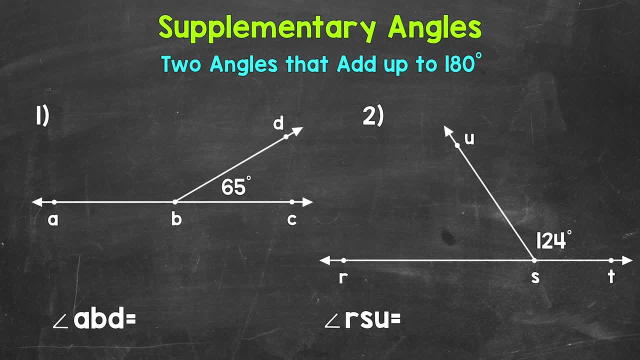 And a 180-degree angle is going to make a straight line. So if the sum of two angles is 180 degrees, they are supplementary. Let's jump into our examples where we have supplementary angles but one of the angles will be unknown or missing. 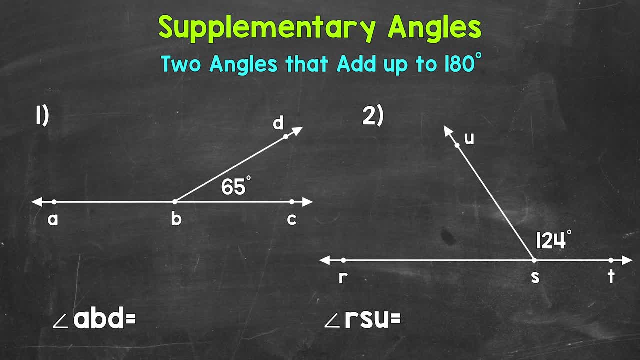 And we need to find that missing angle measure. For number 1, we have a given angle measure of 65 degrees. So angle D, D, B, C equals 65 degrees. So we need to find the missing or unknown angle. 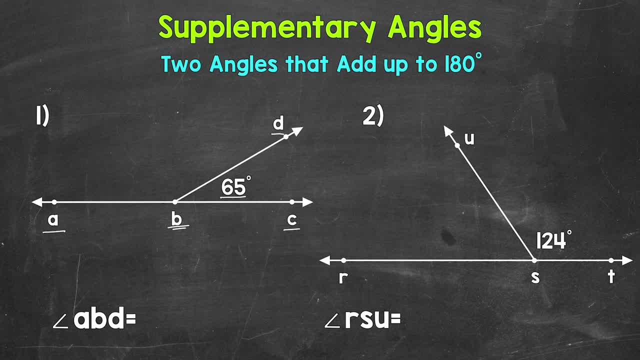 We are going to look for angle A, B, D. Now we know that the sum of these two angles is going to be 180 degrees. They are supplementary angles, So we need to think We have 65 degrees And then we need to add what to get to 180 degrees. 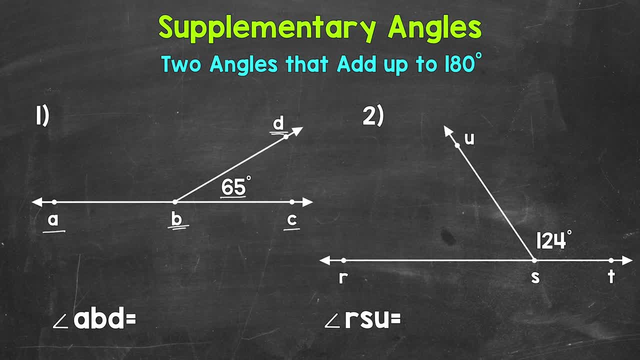 If you can figure these out mentally, that works for sure, But if not, that's fine too. So what we can do, we can take the sum of these two angles, which we know is going to be 180 degrees, So we will write 180 degrees. 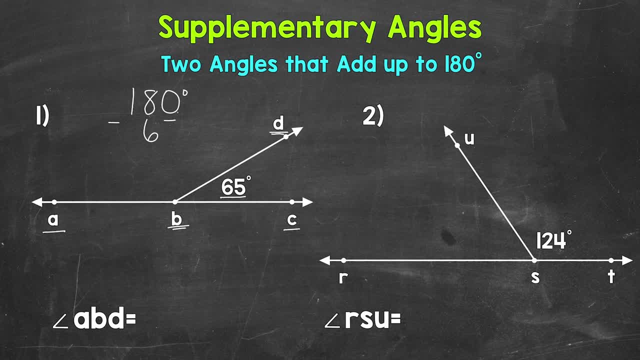 And we'll subtract the angle measure that we are given, 65 degrees. That's going to give us our missing angle. So let's subtract 0 minus 5.. Well, we need to borrow: 10 minus 5 is 5.. 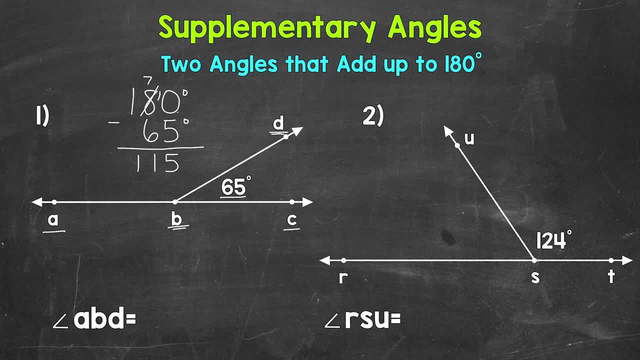 7 minus 6 is 1.. And then we have a 1 in the hundreds place, So 115 degrees, And that is angle A, B, D, 115 degrees. We can always double check our work and make sure that that angle measure is correct. 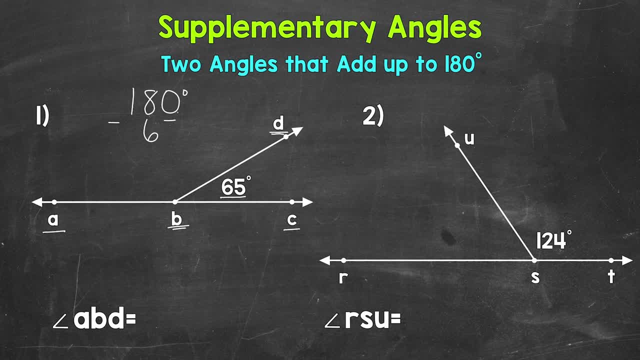 And we'll subtract the angle measure that we are given, 65 degrees. That's going to give us our missing angle. So let's subtract 0 minus 5.. Well, we need to borrow: 10 minus 5 is 5.. 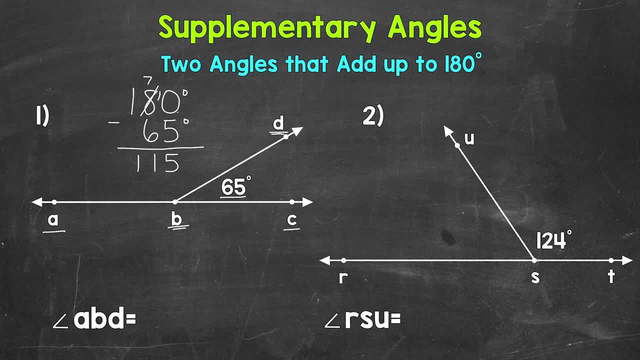 7 minus 6 is 1.. And then we have a 1 in the hundreds place, So 115 degrees, And that is angle ABD: 115 degrees. We can always double check our work and make sure that that angle measure is correct. 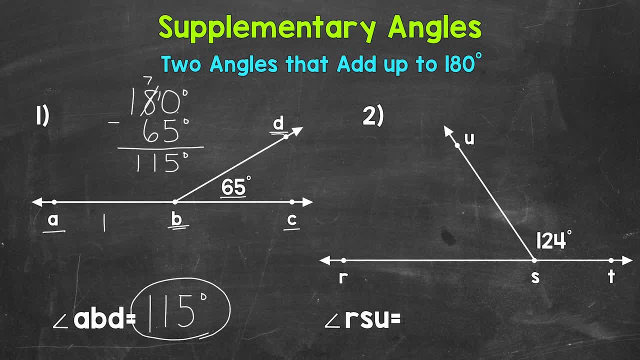 And we do this by adding 115 degrees plus the 65 degrees And make sure they equal 180.. We'll start with 5 plus 5, which is 10.. We'll put our 0 here, Carry the 1.. 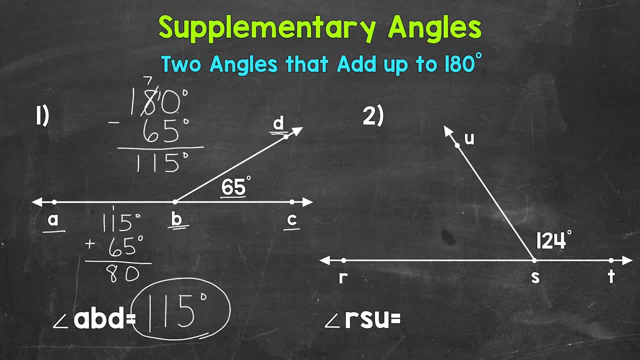 1 plus 1 is 2.. Plus 6 is 8.. And then we have a 1 in the hundreds place. So 180 degrees, 115 degrees was correct And we are good to go. Let's move on to number 2, where we have a given angle measure of 124 degrees. 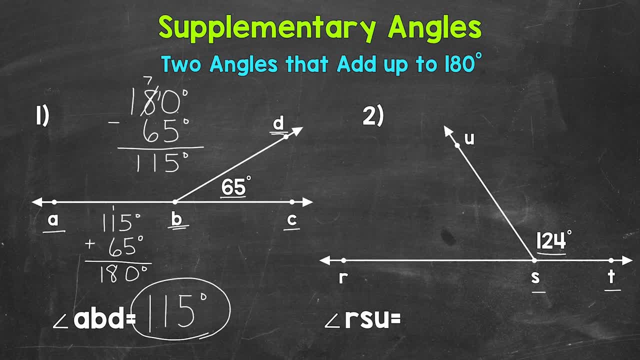 So that's for angle TSU. So with that given angle we need to find the angle measure of angle RSU. Let's calculate what that missing or unknown angle measure is by taking 180 degrees and subtracting our given angle measure of 124 degrees. 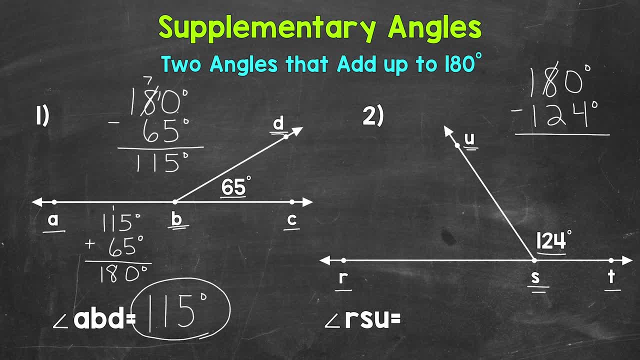 So we'll start with 0 minus 4.. We need to borrow. So we have 10 minus 4, which is 6.. 7 minus 2 is 5., And then 1 minus 1 is 0. So we have 56 degrees. 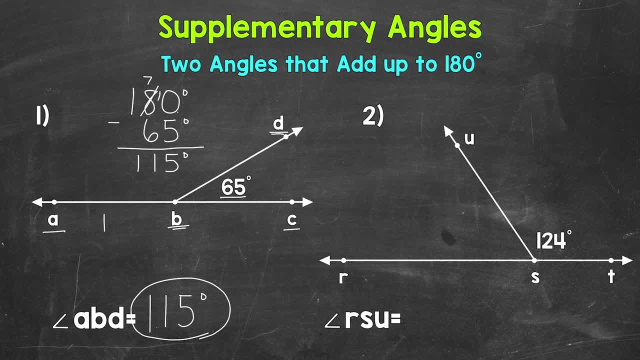 And we do this by adding 115 degrees plus the 65 degrees And make sure they equal 180.. We'll start with 5 plus 5, which is 10.. We'll put our 0 here, Carry the 1.. 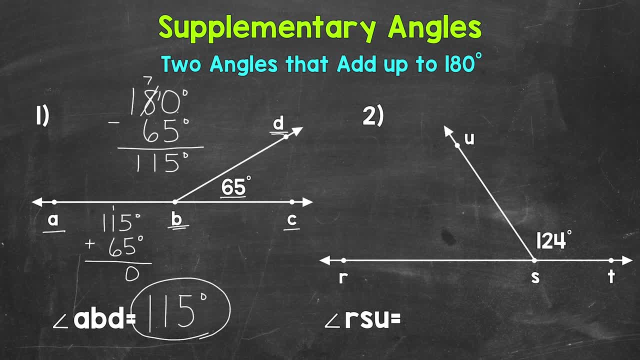 1 plus 1 is 2.. Plus 6 is 8.. And then we have a 1 in the hundreds place. So 180 degrees, 115 degrees was correct And we are good to go. Let's move on to number 2, where we have a given angle measure of 124 degrees. 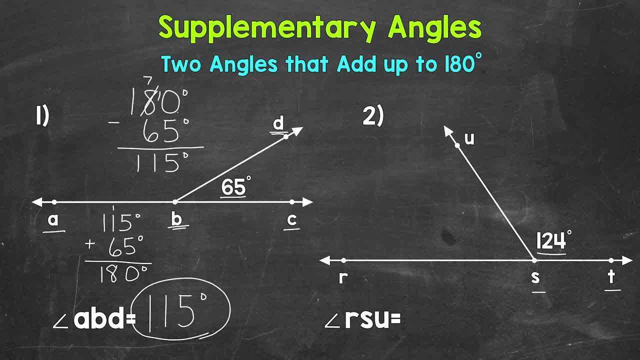 So that's for angle T S U. So with that given angle we need to find the angle measure of angle R S U. Let's calculate what that missing or unknown angle measure is by taking 180 degrees and subtracting our given angle measure of 124 degrees. 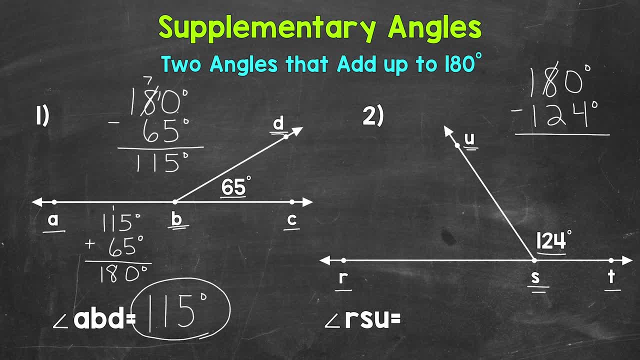 So we'll start with 0 minus 4.. We need to borrow. So we have 10 minus 4, which is 6.. 7 minus 2 is 5., And then 1 minus 1 is 0. So we have 56 degrees. 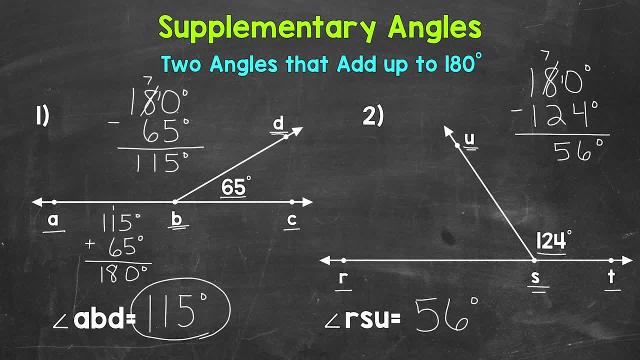 Angle R S? U equals 56 degrees And again, we can always double check. Let's do that So we can add 124 degrees plus 56 degrees And make sure that equals 180 degrees. 4 plus 6 gives us 10.. 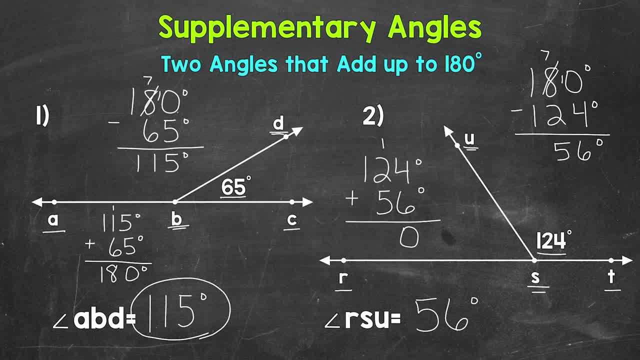 Carry the 1.. 1 plus 2 is 3. Plus 5, 8. And then we have a 1 in the hundreds place. So 180 degrees, 56 degrees was correct for angle R S? U. 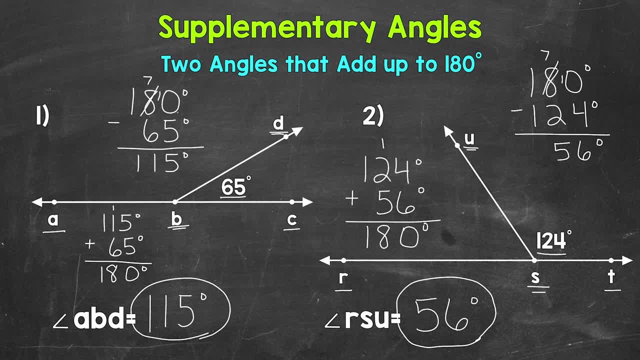 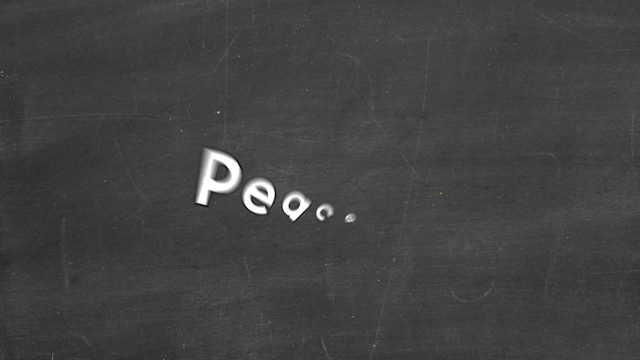 So there you have it. There's an explanation of both complementary and supplementary angles And how to find missing complementary and supplementary angles. I hope that helped. Thanks so much for watching. Until next time, peace.